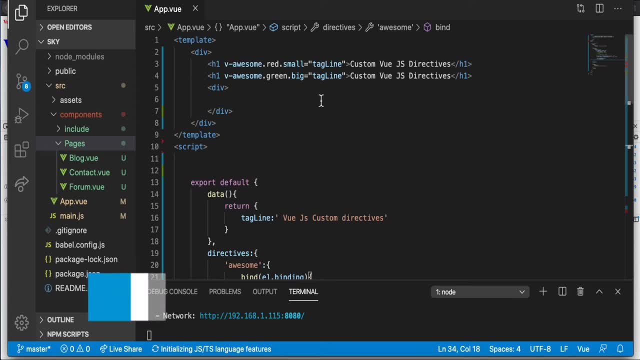 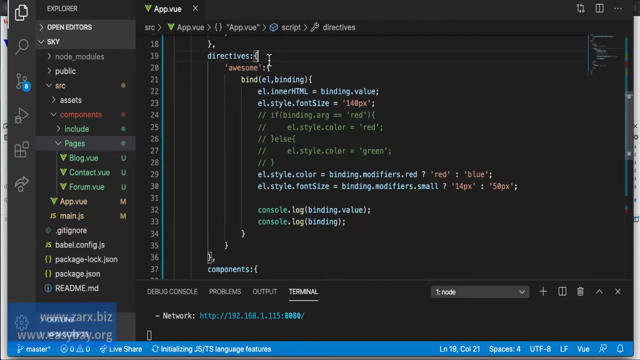 Welcome guys, welcome to this brand new VJS video. So in last video we talked about the custom directives and in the custom directives I talked about how we can define custom directive globally as well as locally. We did that and we are now going to talk about the hooks. hooks function in the custom directive. So we created this directive with the name of awesome and I already used one hook, which is bind. 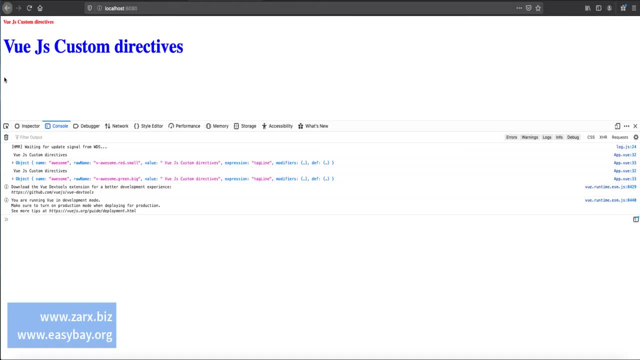 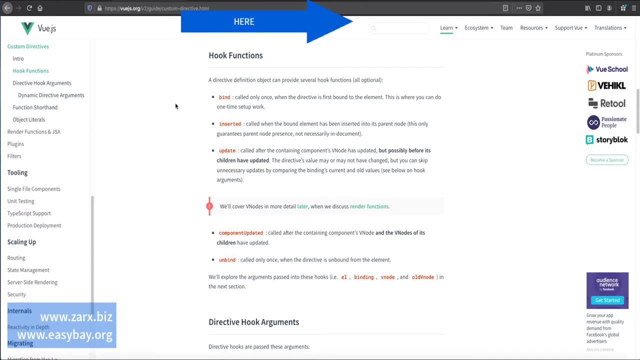 Now there are more hooks. if we go to the documentation In custom directives there is hook functions. We have bind. we already saw it in the previous video- If you haven't seen that video, you should check that- And then we have inserted, we have update, we have component updated and unbind. 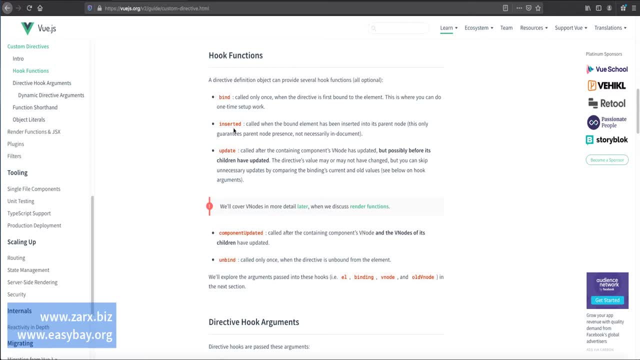 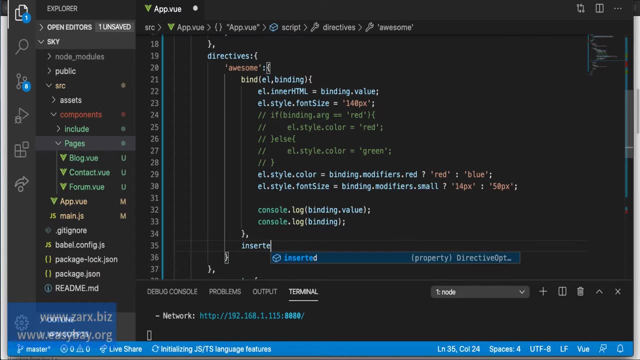 So let's see the difference between bind and inserted. So if I go to the code here and here I say inserted, So by default all the hooks get the values, these arguments, So I can use the same arguments in here. Now if I want to check the parent node, parent element of the div or whatever HTML where I am including my directive, this custom directive, 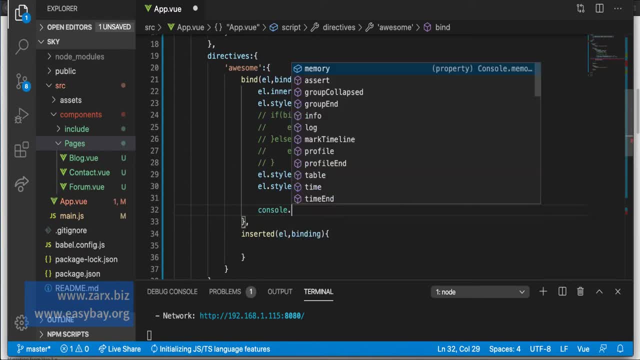 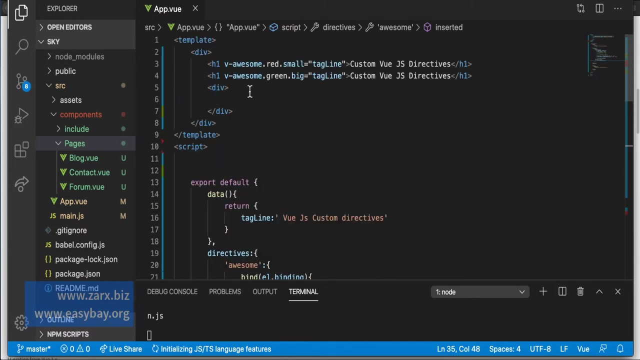 So I can put here console dot log and then element dot- parent node. So it should return the parent node. So what I am going to do, I am going to copy the same console dot log in here. Now we are using this custom directive twice on the same page. If I go here on the top, you can see I am calling this here as well as here. 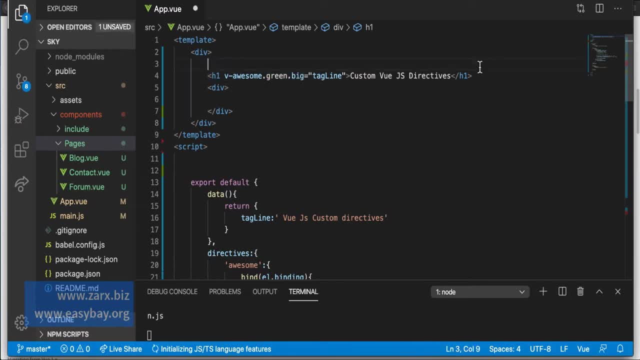 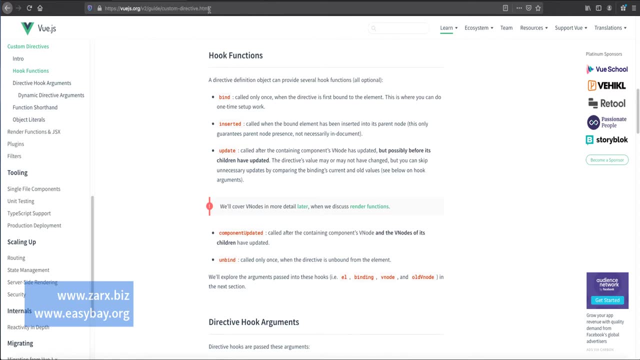 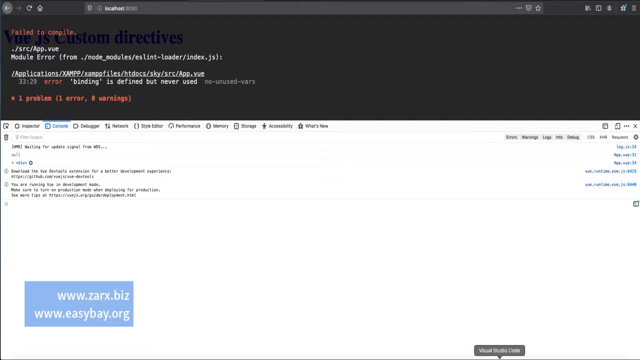 So what I do? I am going to remove the one on the top, Alright, so save that. If I go to the code and on our site, if I refresh the page, It says binding is defined but never used. So if we are not using the binding, it returns the error like this: 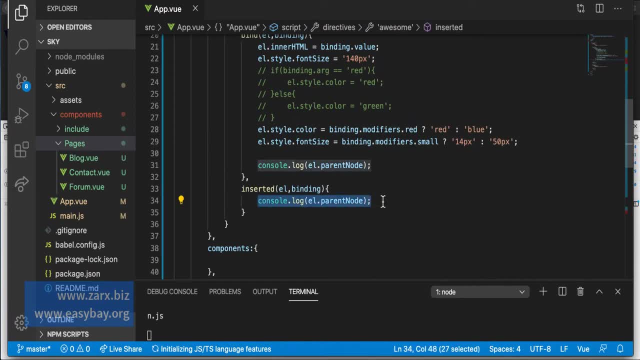 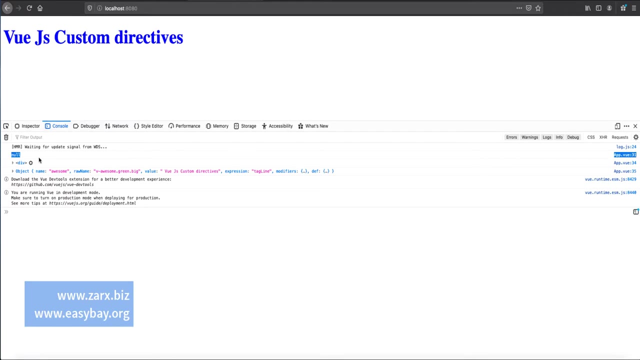 So what we can do in this case? just copy this one more time And just use the binding. I am just going to paste it here so that the error goes away. Alright, so we get this. So here we are getting null as well as div. 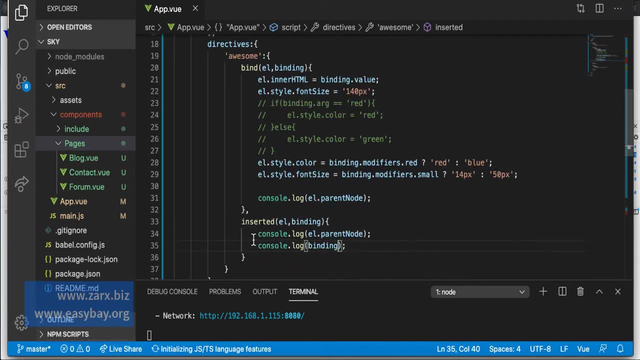 So if you go to the code, What happened is inserted is going to run once the DOM is ready. DOM is the document object model, So the bind is runs when your custom directive binds itself to the element, So it runs before it. That is the reason we get null. 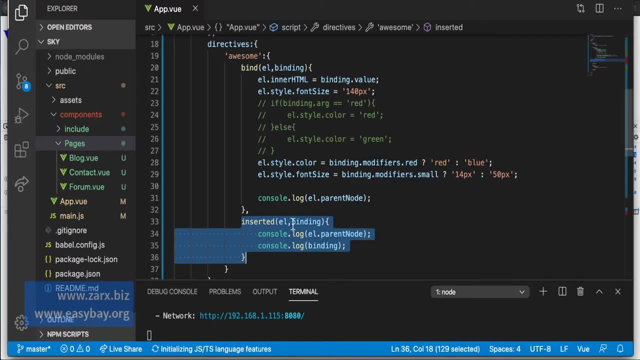 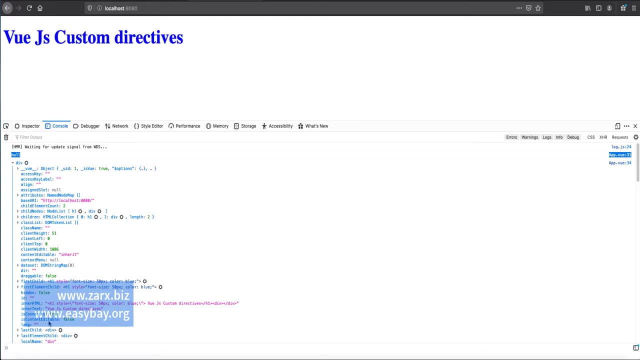 Now the inserted inserts inside the DOM, So that is the reason we get the parent element of div And we can access so many values in here. you can see Now if I go here and if I comment this And save it. Refresh the code. 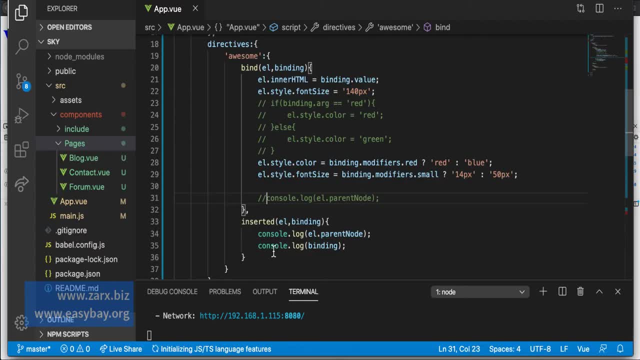 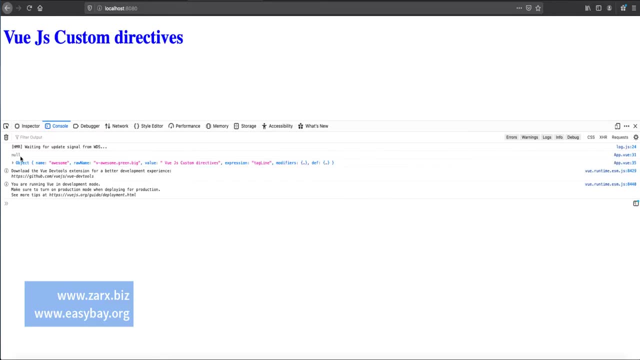 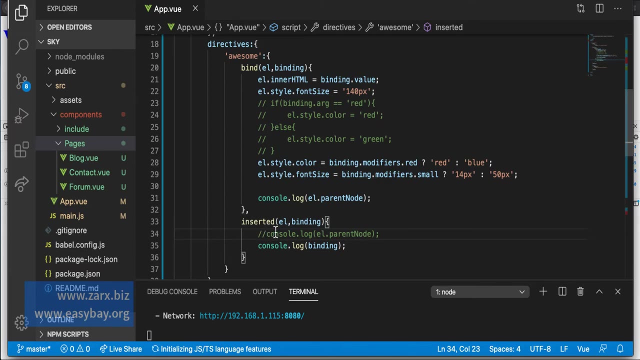 We won't see the null because it is not firing from the bind. And if I show this and hit save and refresh, Now we have null and we are not getting the parent div. You can see there is no div element. So that is how this is working. 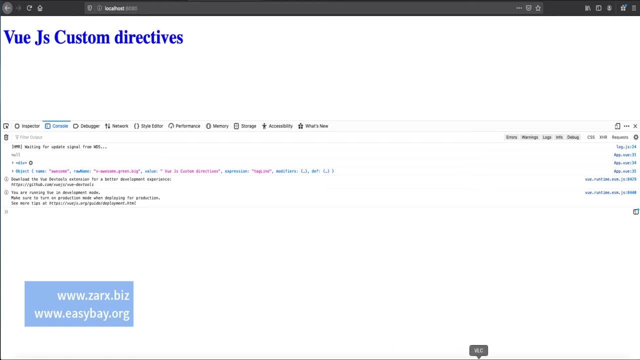 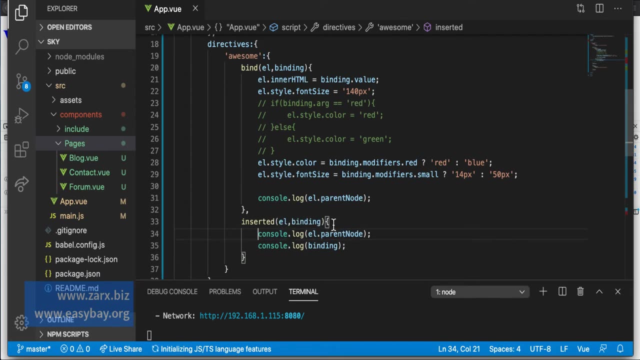 So whenever you use, You can use The inserted. whenever you want to do something, Once the document is ready, You can use it. You want to access it in a particular tag, Then you can work along using that, And here you can't do that. 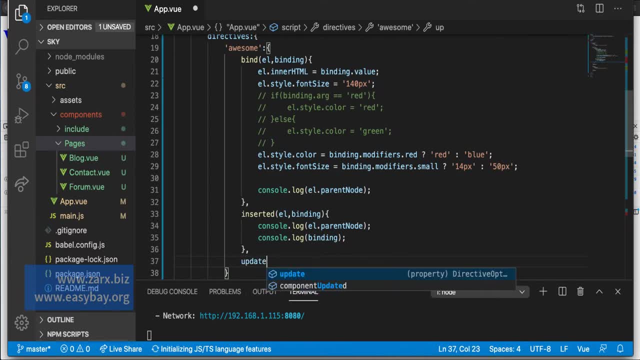 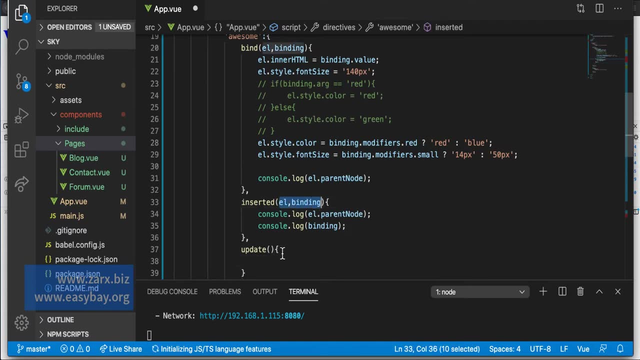 Another hook is update. So to work with that is just type the update function And we get the same arguments. We can use the element bind in this one as well, So we can put that in here. So update fires whenever you are going to update something. 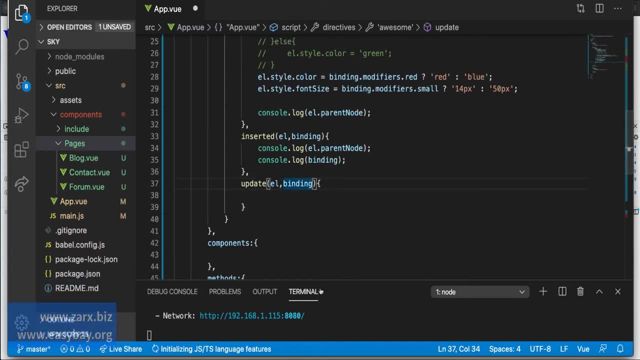 Otherwise it won't fire. In update we get the third vnode as well, As well as we get the old vnode. So vnode is something that we are going to use very rarely, Because in real life projects vnodes are used rarely. The difference between vnode and old vnode is: 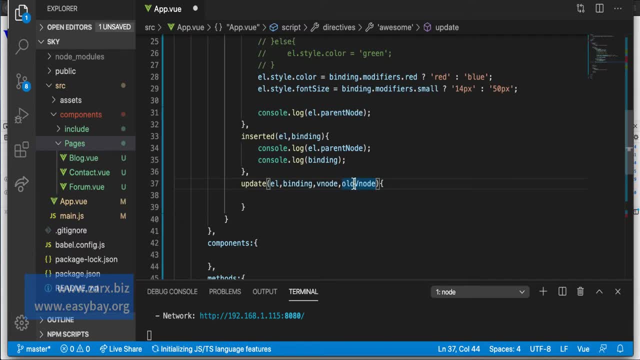 When update happens, It is going to give you the old values And it is going to give you the updated values. What I do straight away? I just connect, Comment this And copy comes along here And I am going to put all these values too. 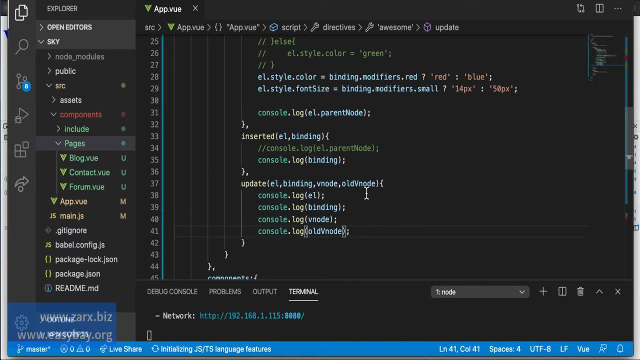 And then put old vnode here. I save this. It is not going to do anything Because if you go refresh it is not going to show up. The reason is because it is going to fire only on update. So to do that what I do, 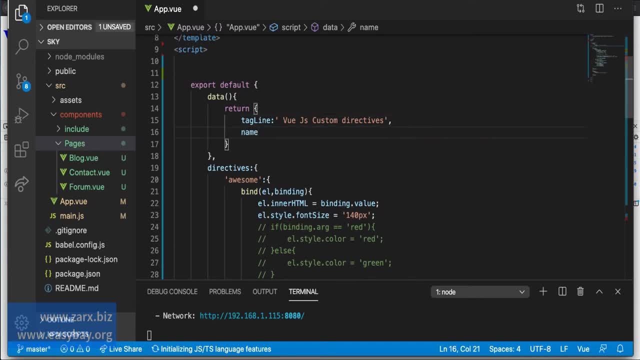 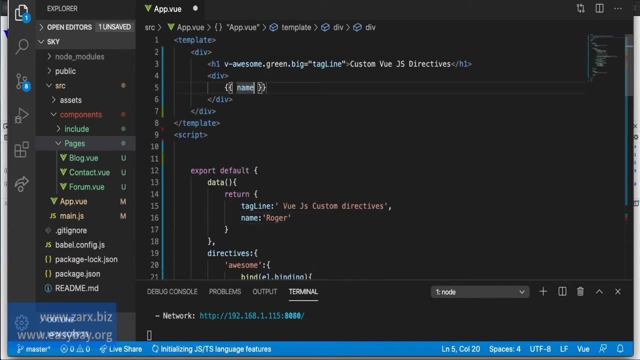 I create a property And we will update that property. So I say name And by default I say it is launcher. Now we can display this name, Say here name And to update it In the created lifecycle method I say set timeout. 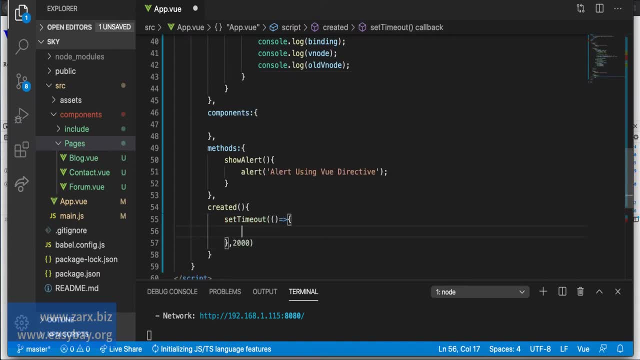 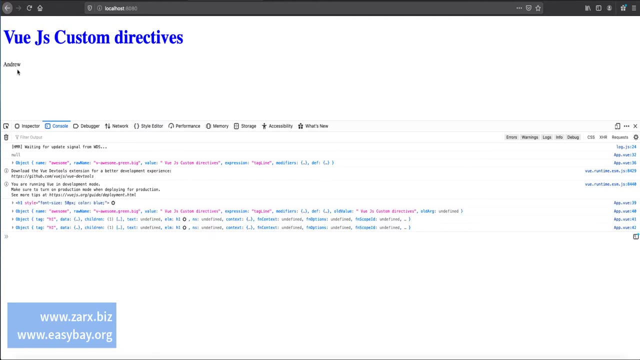 Let's say two seconds, And what I want to do Is this dot name Is equal to: Let's say Okay, So Let's save that, Refresh the page And we get the interview. Now we also get the output. 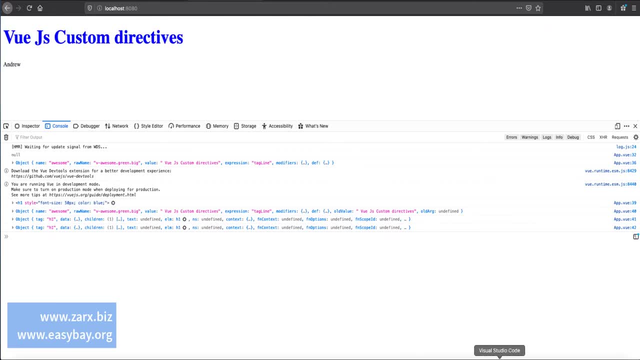 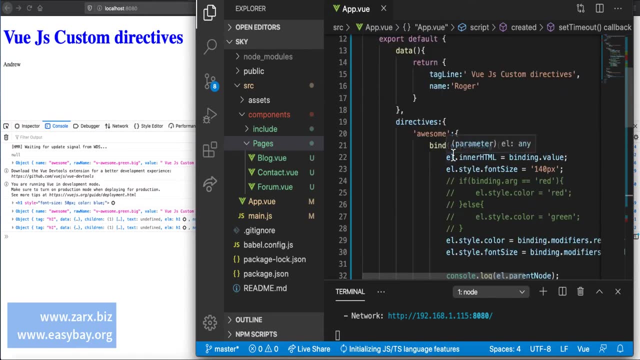 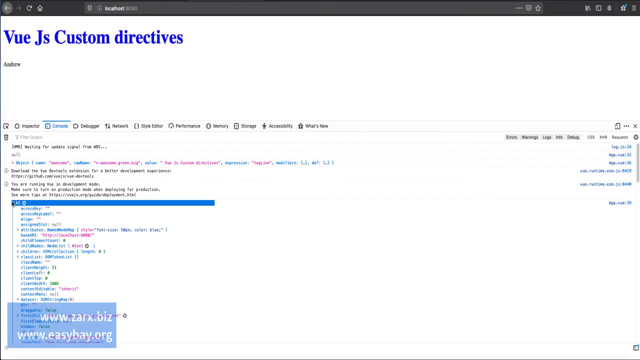 Now, if you see here We get four If I go to the code. The first one is element, The element we call this custom directive on. So we call it on h1. So we can get the h1 here. We can select the values using element. 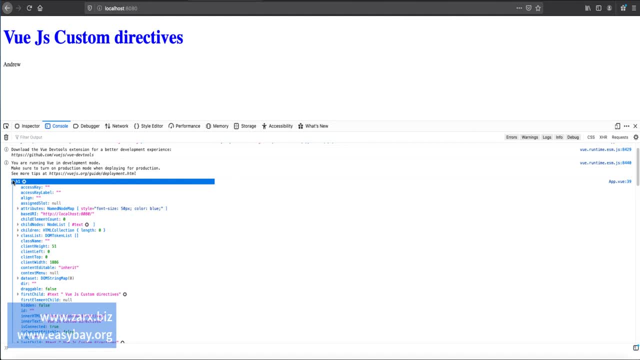 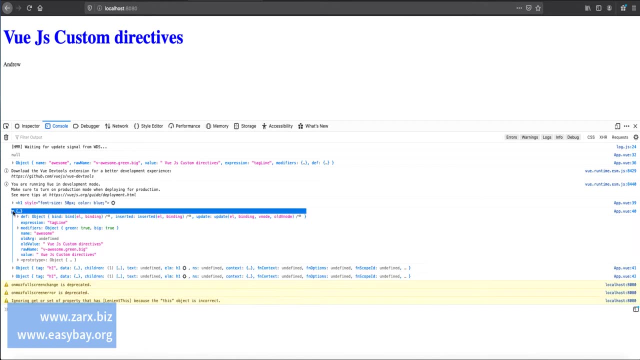 And do whatever you want to do with this. You can do that. The second, If we go to It, is the object. Now, this is the binding object That uses to get the values, So we can use modifiers And expressions. 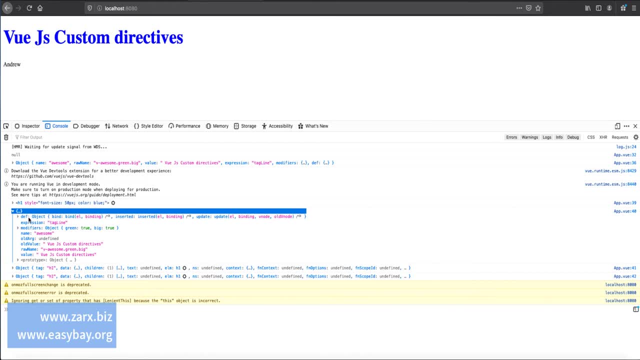 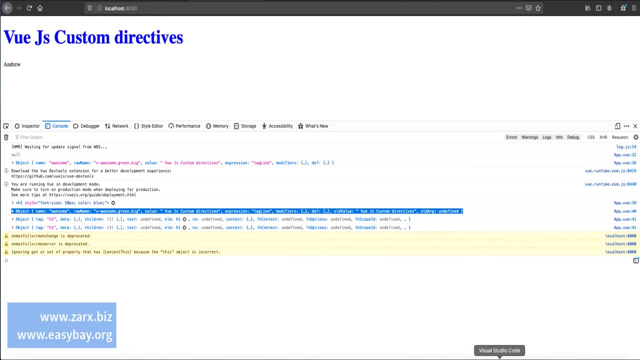 And everything We can Using bind Binding. We can get the values. We already checked that in the previous video. If you Haven't checked that, You should check that video as well. Now here In the third, If I go here, 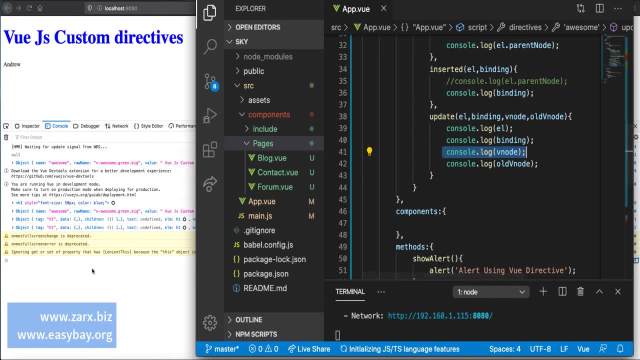 It was v-node. V-node is the updated one, So we have the elements here And it is something that you can use. them If you want to explore, You can check them, But v-node And all v-node Is going to be used very less. 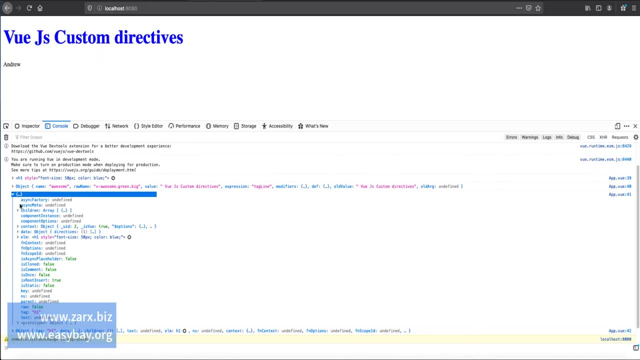 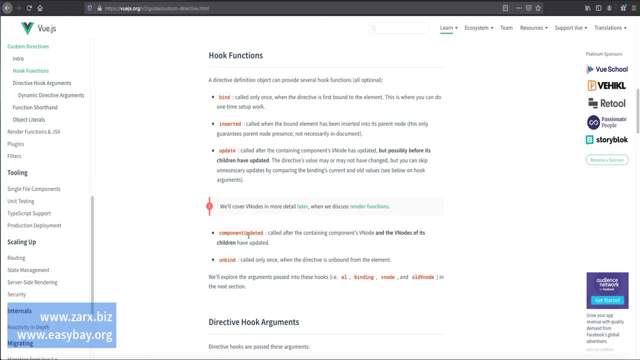 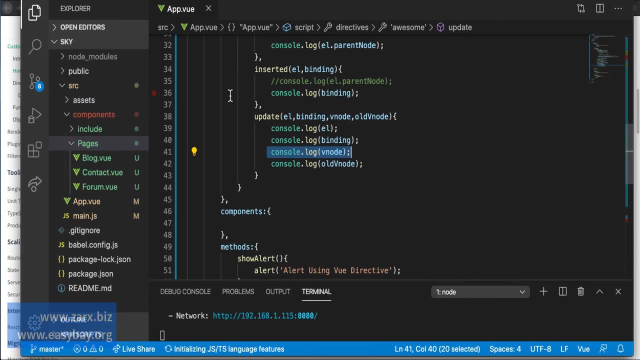 We have the updated And then we have the complete Update. So Copy this, And I am just going to add this as well, With the line: These two And also These here, from here. So And it won't give us the address. 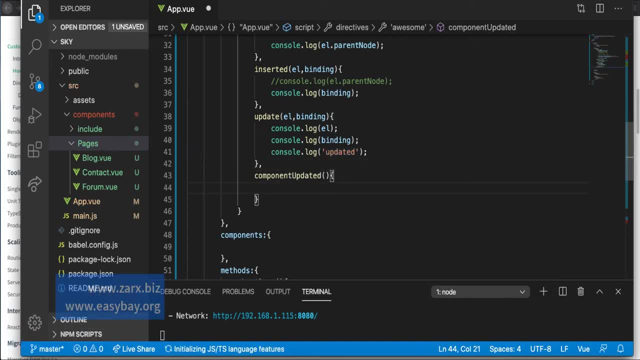 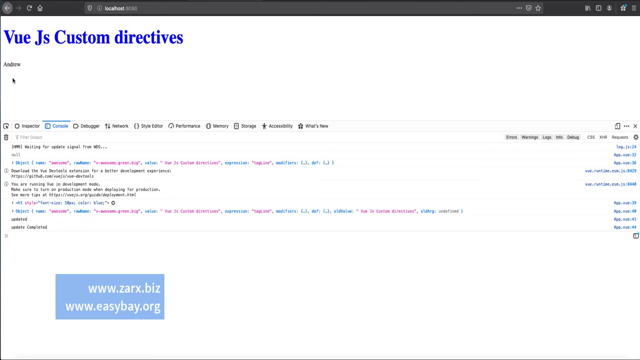 so it's a console dot line line in here. so update completed. so save this and we give to the document again and refresh the page. now we get updated because it updated the value and after that, once updated is completed, we get an update completed. now get the id update completed for us. 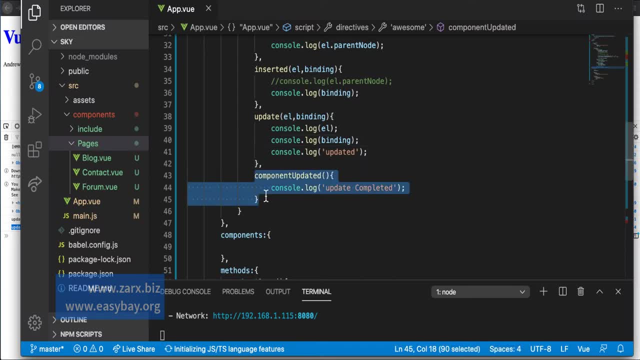 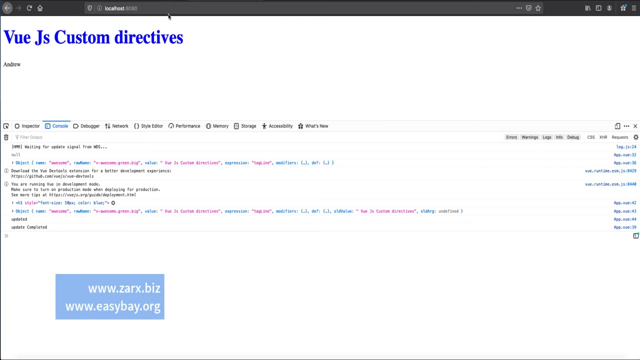 after once the update is completed. now order doesn't matter if you cut this and put it before it. that doesn't going to make any change because, process wise, it is going to work just after the update. so refresh, you will see it in the same manner: updated and then update completed. 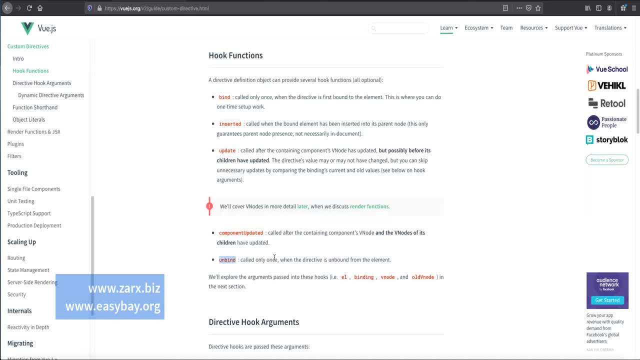 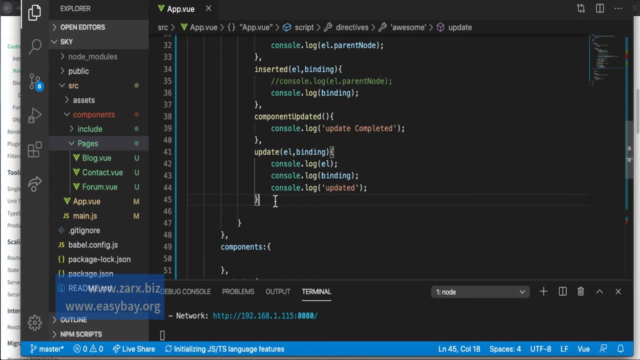 now, other than this, we get the unbind- unbind called once when the directive is unbound from the element, so can you use the same one is here. find now in all these elements there's a button that goes to the address and if you put this in the 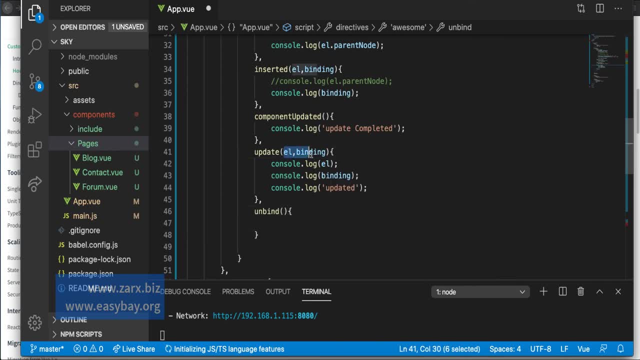 elements. We get all the arguments. as I said, We get the element and binding in unbind as well. We get in complete a bit as well, So we can use them as we want. So here we can say consolelog unbind. So then the element going to be. 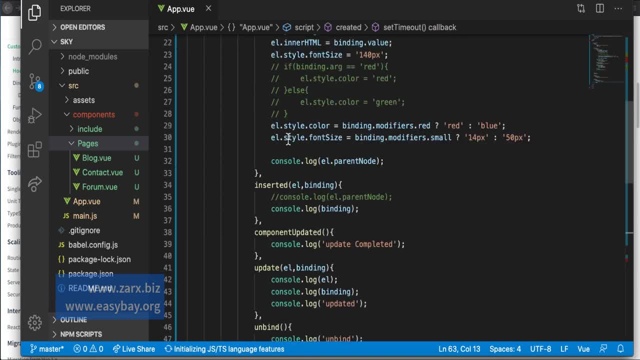 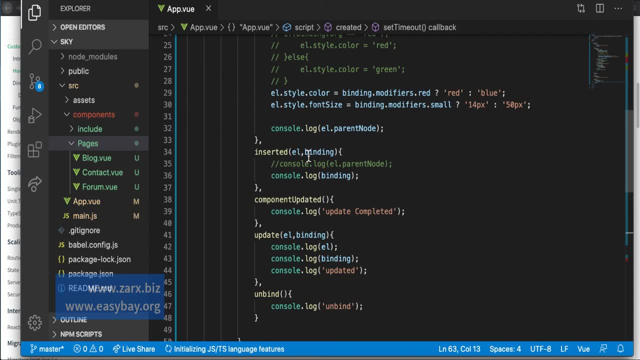 unbind. it is going to fire only once. We are mainly going to use the bind inserted and the update methods functions in custom directives, in the coming videos, as well as in the projects. Unbind will fire when we are going to remove the element from the DOM, So that happens. 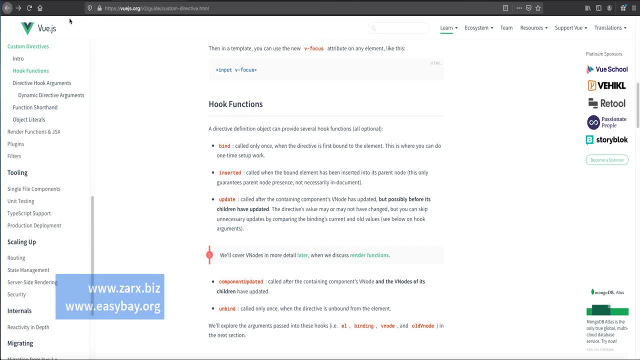 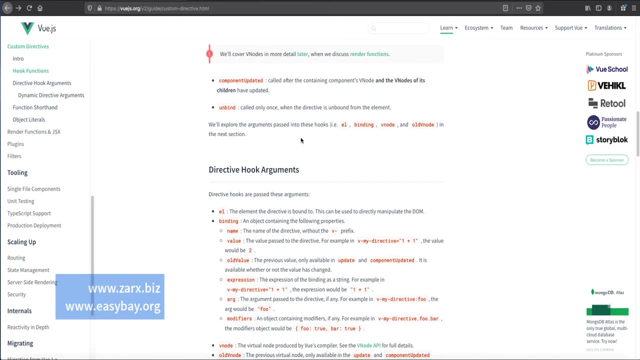 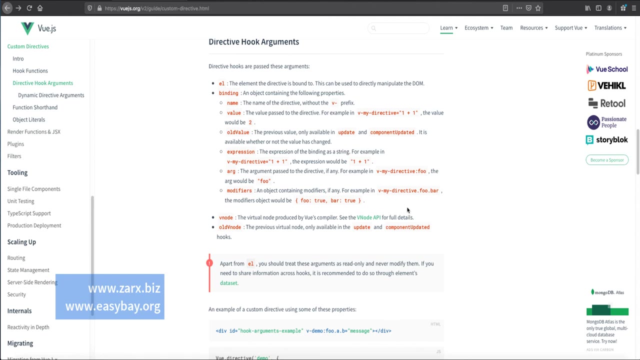 really, and if you want to read more about it, you can go to the documentation, and the link is here. You can read about the functions as well as the argument that we are passing here: the element and binding and bnode and all that. Everything is completely explained here as well. 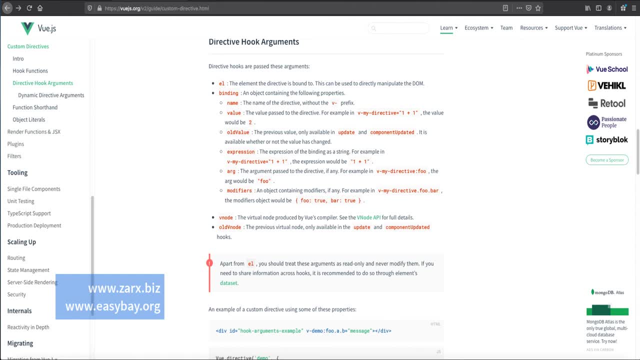 if you want more to explore it more. So if you like the video, do subscribe, share and have a nice day.